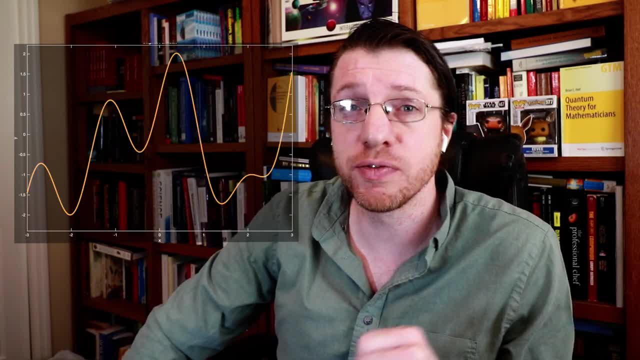 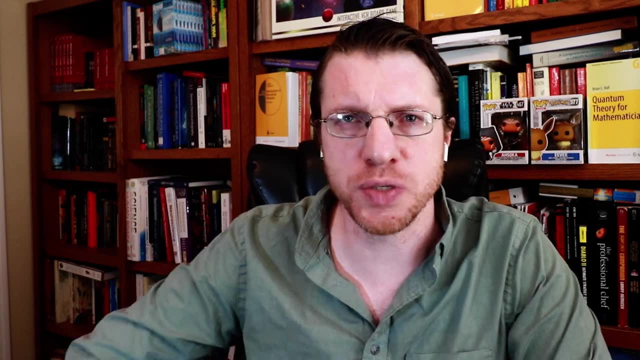 look at a vector space of infinitely differentiable- ie smooth functions- And we're going to define a topology by defining a collection of semi-norms. This is nearly identical to how it's done on the Schwarz space. Now for this discussion. we are going to be following. 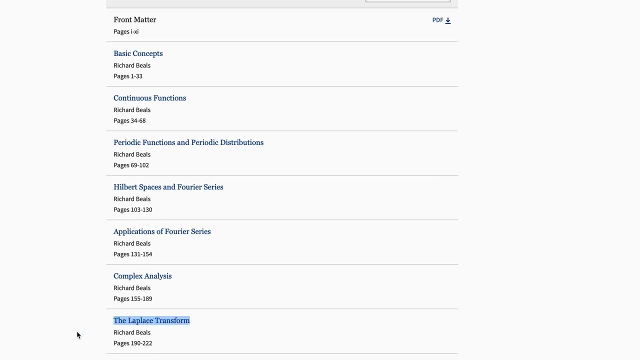 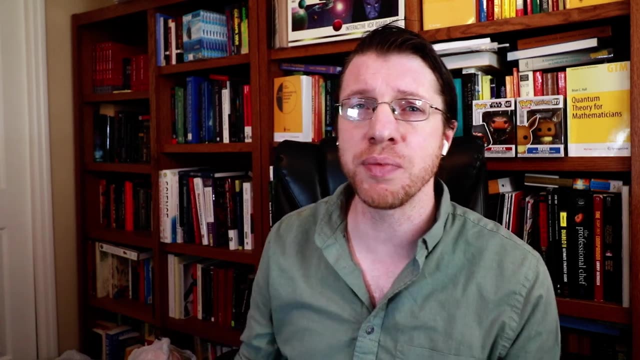 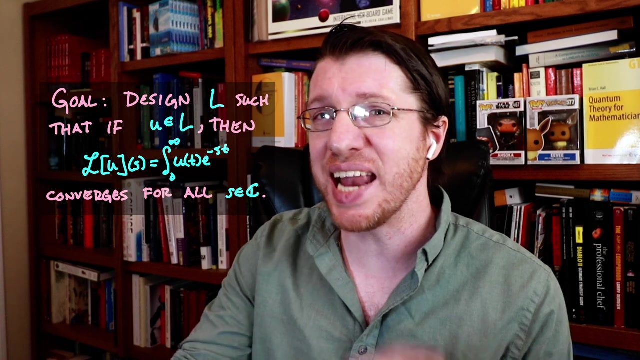 Biel's text Advanced Mathematical Analysis because I felt the presentation there was a link to that book in the description. The ideas behind these definitions all stem from the Laplace Transform definition, where we want to make sure that these functions have a well-defined Laplace Transform, given any s in our complex plane. Now there are more. 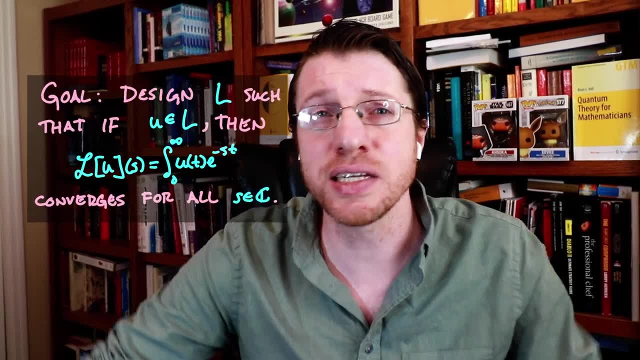 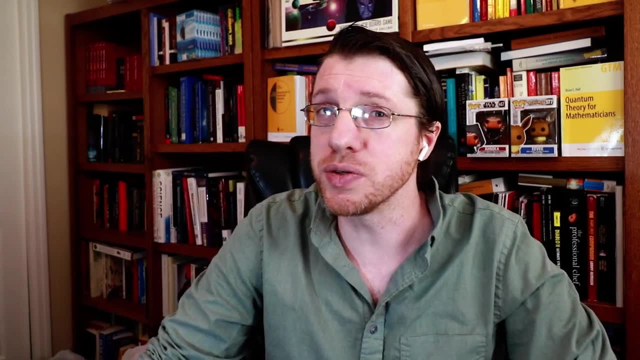 Laplace Transformable functions than these. but our goal is not to define the Laplace Transform on these functions, but rather on the continuous functionals of these functions, which includes the Delta function. Now take a smooth u that maps the reals to the complex. 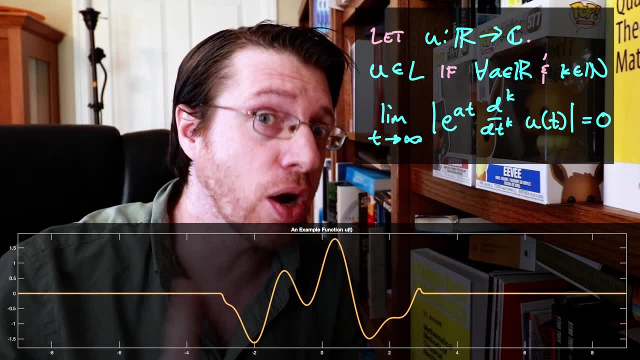 plane. Now take a smooth u that maps the reals to the complex plane, such that for every k, such that for every k, such that for every k bigger than or equal to 0, and a and r the limit as t goes to. 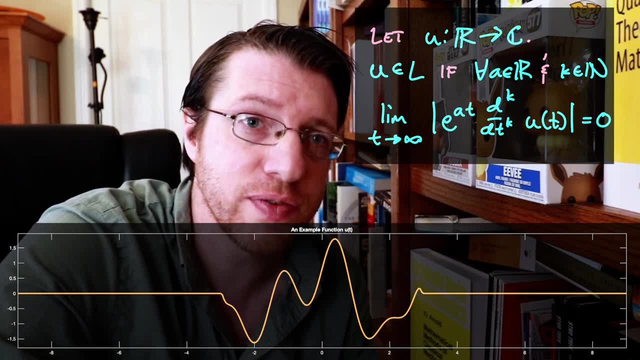 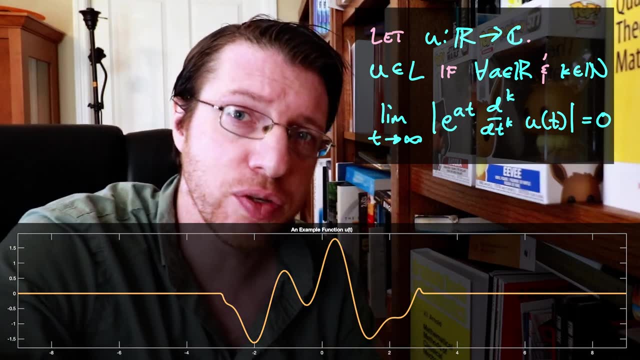 infinity of e to the a t times, the kth derivative of u of t goes to 0.. It turns out that this is a vector space, which we will call L, and this follows, since all of those operations are linear. Moreover, we define a topology on this space through a collection of what 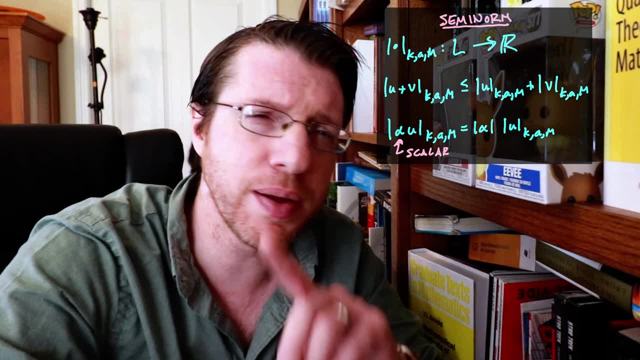 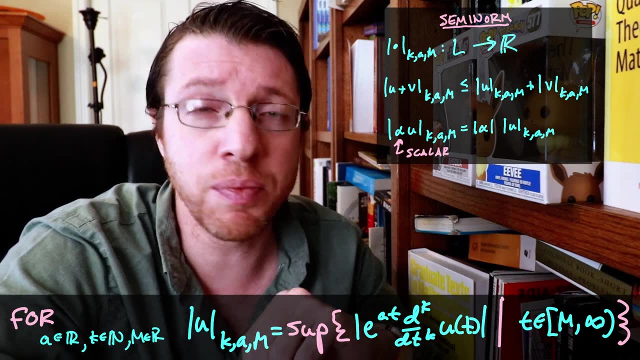 are called semi-norms, which are individually very close to a norm, with the key difference that they send more than one function to 0.. These are as so. where we take m to be any number in R, Note that they satisfy a triangle inequality and you can pull scalars out at. 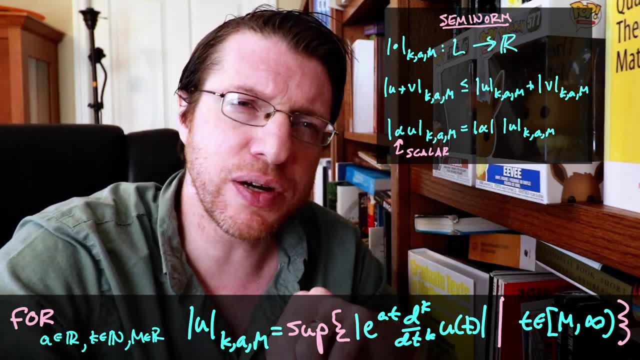 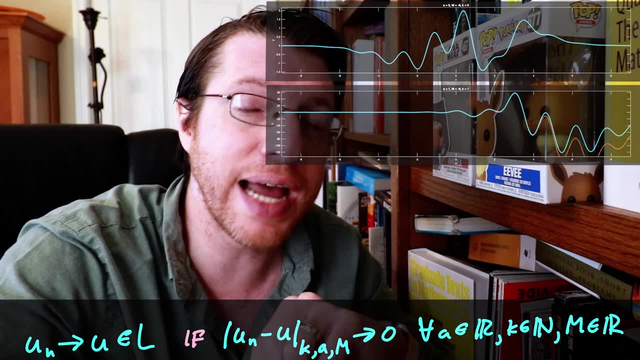 the cost of an absolute value. We say that a sequence of functions in L converges to another function, u in L, if the difference under each semi-norm goes to 0, as n goes to infinity. Conversely, we have a Cauchy sequence if the difference between two elements of 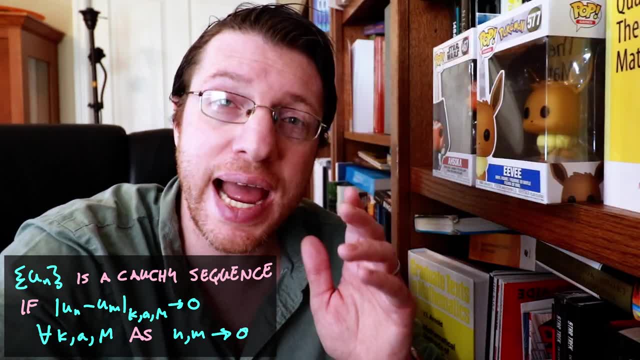 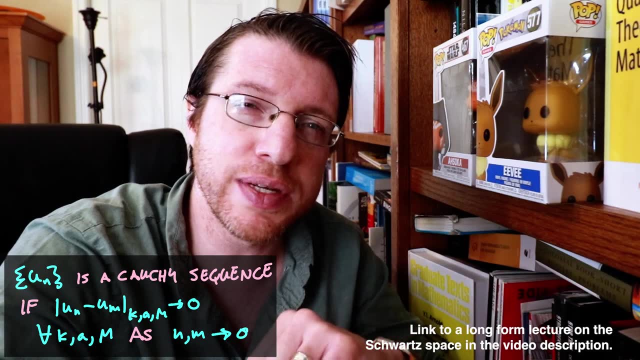 the sequence goes to 0 under each semi-norm, as n and m go to infinity. In fact, L is complete and you can see that each Cauchy sequence is equal to the number of semi-norms. that is a convergence sequence. in the same way, 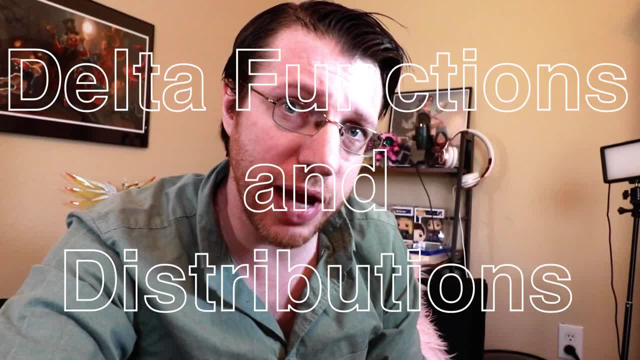 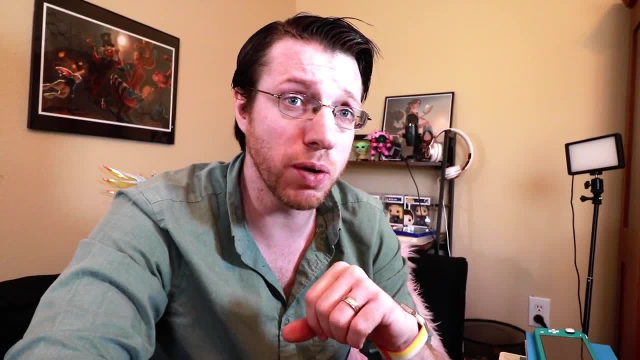 that is done for the Schwarz space. So now that we have a topology, we can talk about closeness And in turn, we can talk about continuous mappings, where small changes in the input lead to small changes in the output, And one example of these continuous mappings is: 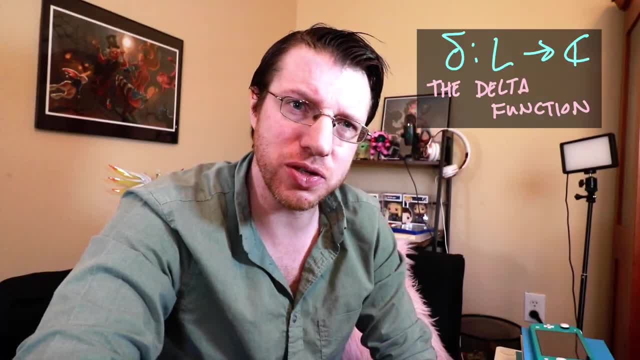 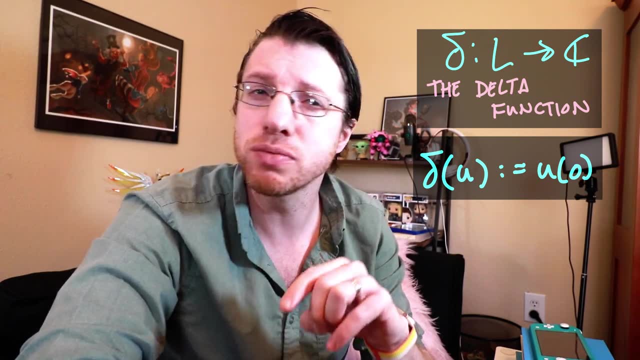 well, you guessed it: the delta function. If we look at the delta function, which takes a function, u to its evaluation at zero, this is a functional that is mapping functions in L to the complex plane, While delta functions manifest as functions over reproduced kernel Hilbert spaces. 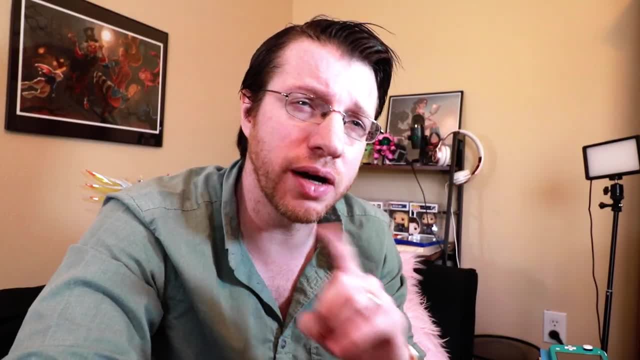 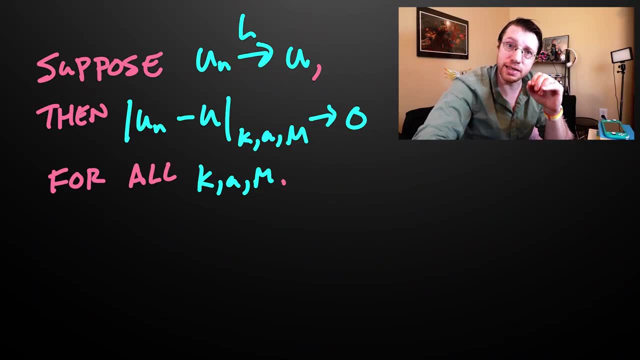 that isn't gonna be the case here, since the shape of functionals really depend on the space in question. Now, if we take a sequence of un's that are converging in L to some function u, then that means that the difference under each semi-norm is going to zero. 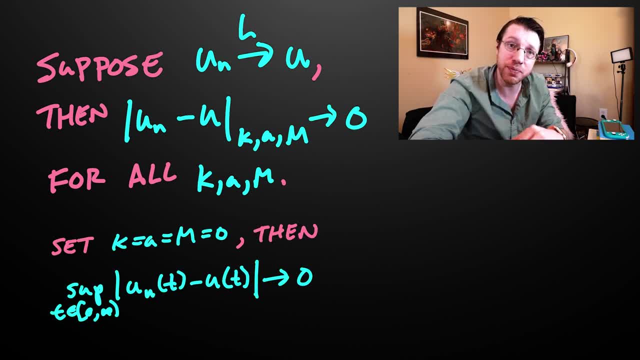 Now, if we set k equals zero, a equals zero and m equals zero, then we have that the supremum of the absolute value of the difference between un and u over the reals goes to zero. And in particular, if we take a look, 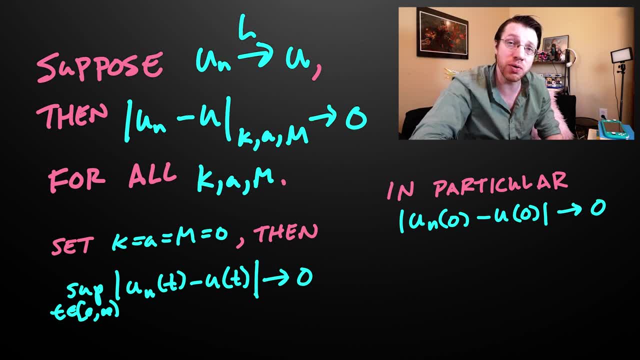 at the zero point, the difference between un of zero minus u of zero in absolute value also goes to zero. Hence delta un converges to delta u. This means that the delta function is continuous over the topology derived from our semi-norms. 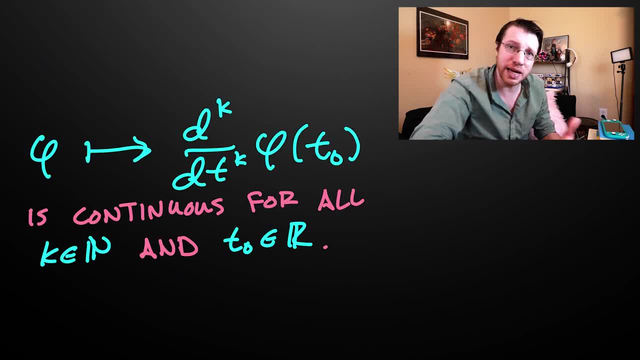 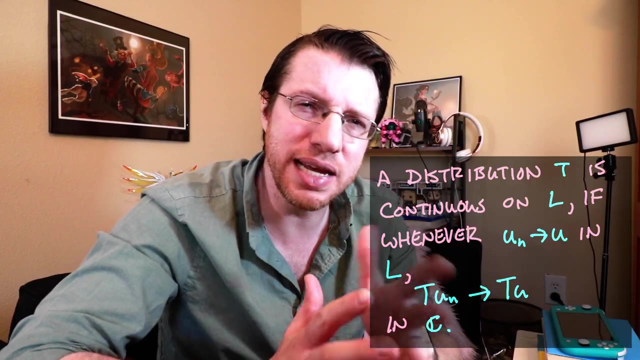 And we can also show that the functionals that map functions in L to the evaluation of their derivatives at the origin or any other point, are continuous in the same manner. These actually turn out to be derivatives of the delta function in some generalized manner. Take a functional t. 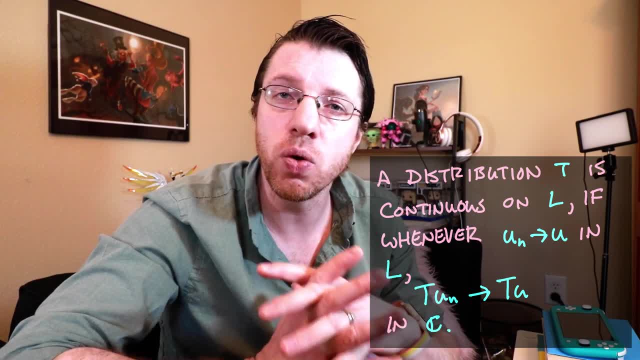 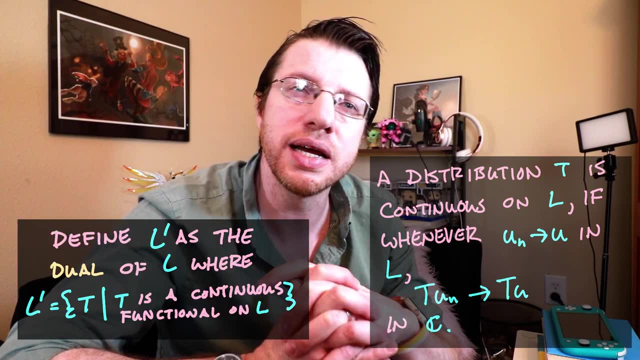 which is a map from a vector space to the space of scalars. We say that a linear functional is continuous over L. if, whenever un converges to u in L, then tun converges to tu in C, While the delta function can't be represented by a function. 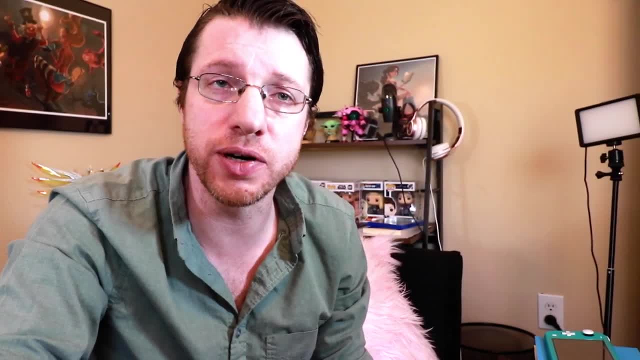 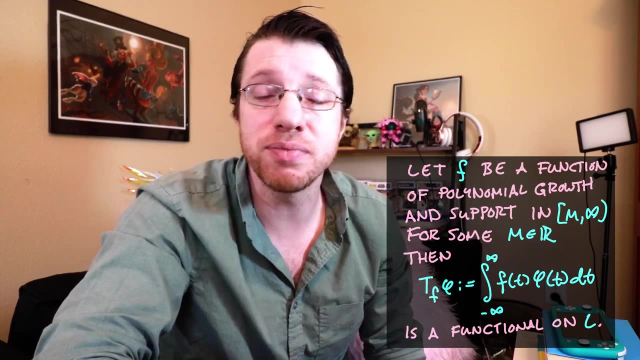 many functionals can. In particular, we call these regular functionals. These manifest by taking a function f of, say, polynomial growth and multiplying against a function in L. Then we integrate them into a function f. We integrate from minus infinity to infinity. 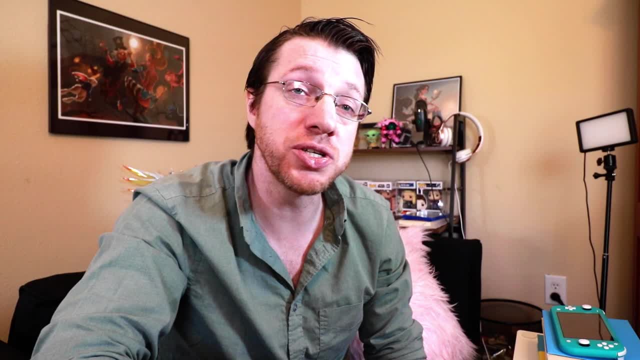 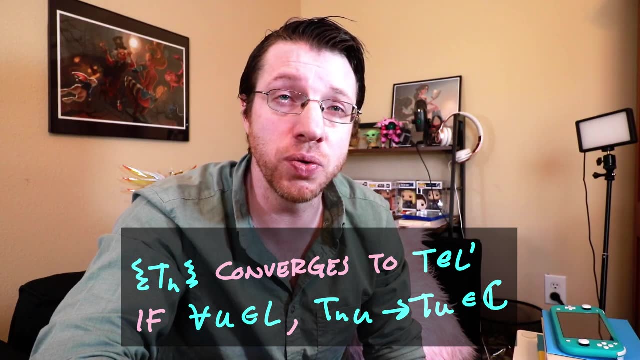 We define convergence of sequences of functionals and hence a topology on the dual space, point-wise, That is, tn converges to t. if the sequence of complex numbers t and u converges to tu for every u, It turns out that every distribution can be expressed. 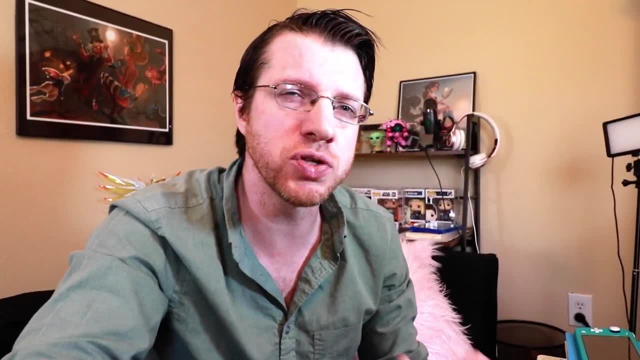 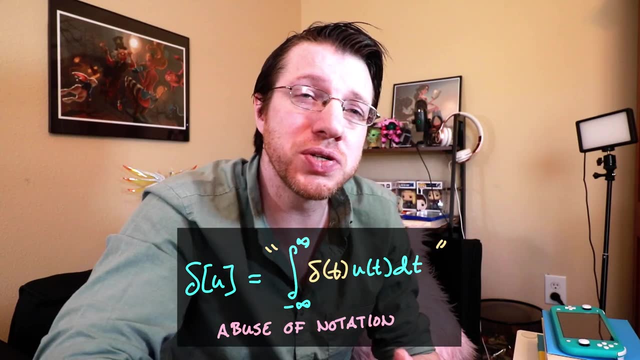 as a limit of regular distributions, which motivates the abusive notation that everybody is familiar with, where we define the action of the delta function through an integral. Now what we do is we actually extend this abuse to all distributions. For a given distribution, t. 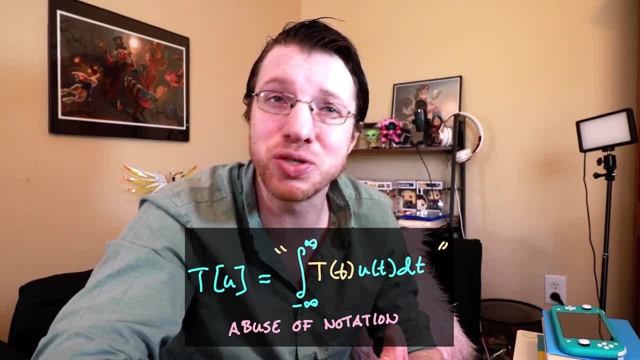 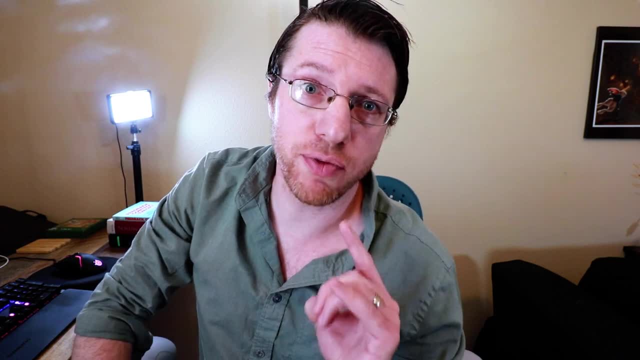 we write its action on u as an integral, and this leads us to the Laplace transform. Now let's give a rigorous definition of the Laplace transform. We know that for an ordinary function on the half line, which is of order one, 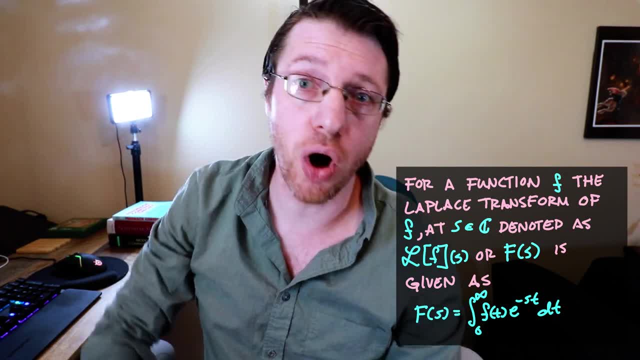 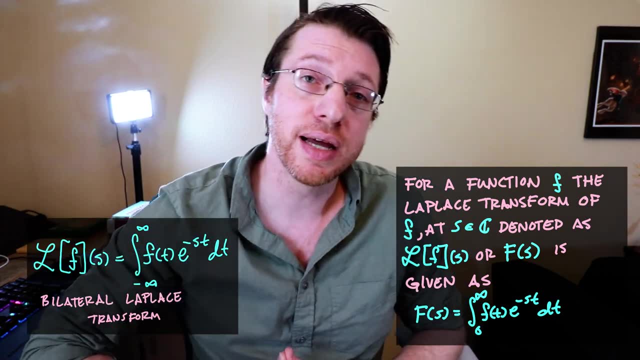 this integral converges for sufficiently large s, We call this the Laplace transform of f at s, and then for the bilateral Laplace transform, we extend this integral to include the left half of the real line. We extend this to distributions. Now, going with the abusive notation, 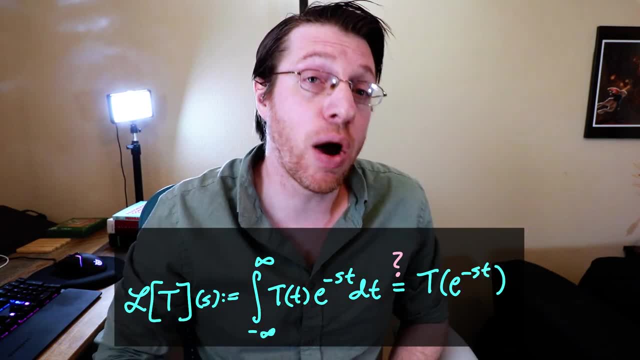 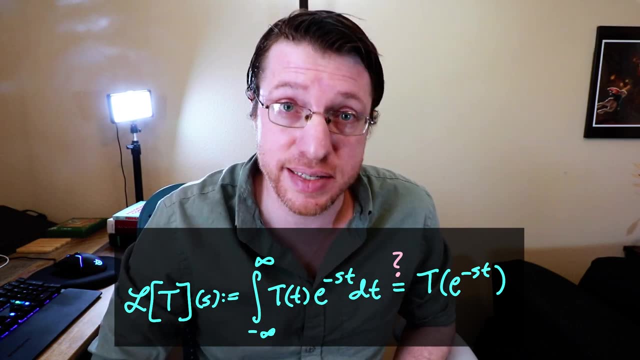 we can write the Laplace transform of a distribution like this. However, we should be aware that this is not an actual integral. It is our distribution acting on e to the minus s t. Rather, we would like it to be, but e to the minus s t isn't in L for any s. 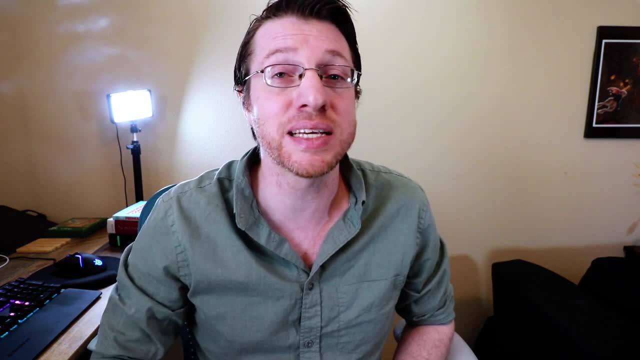 so we need one more step, and that is to approximate e to the minus s t. with functions in L, It turns out that for any s we can get a close up view, and then we can write the Laplace transform of a distribution like this: 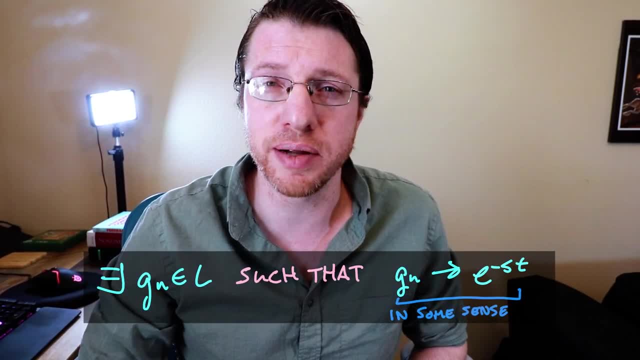 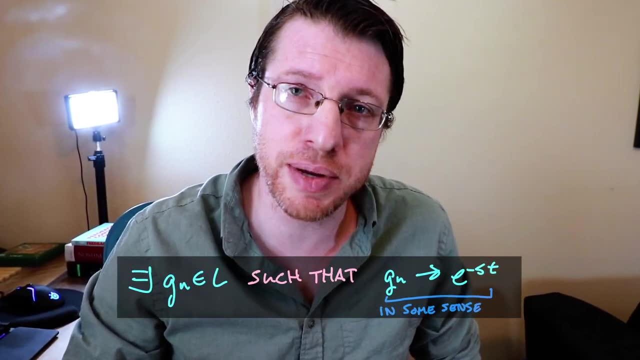 A close approximation of e to the minus s t with functions of L, where the difference between e to the minus s t and a sequence of functions in L goes to zero, according to our collection of semi-norms. where we restrict these semi-norms? 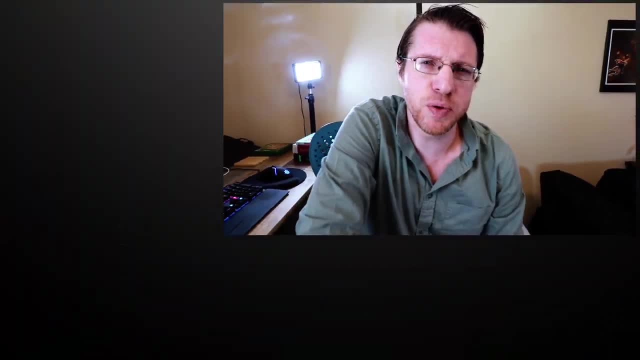 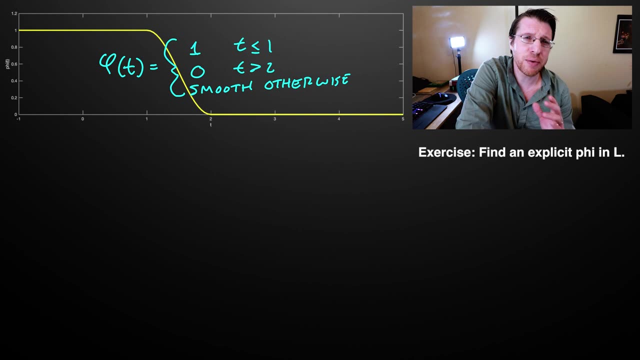 to those where the real part of s is bigger than a. We can do this by taking a smooth function, that is one for t less than or equal to one and zero for t bigger than two, and we'll call this function phi. Then we make our sequence of functions. 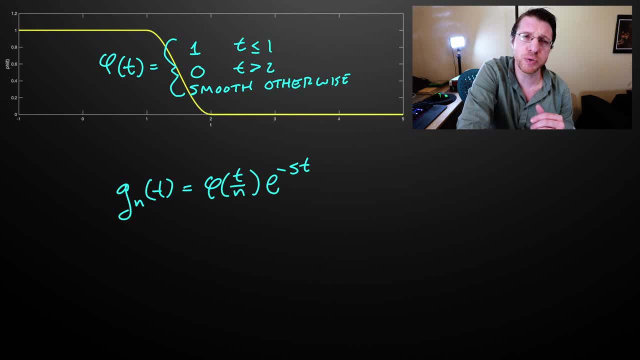 that are gonna approximate e to the minus s t by defining g: n is equal to phi of t over t, t over n times, e to the minus s t and this ends up converging to e to the minus s t. The Laplace transform of a distribution at a point s. 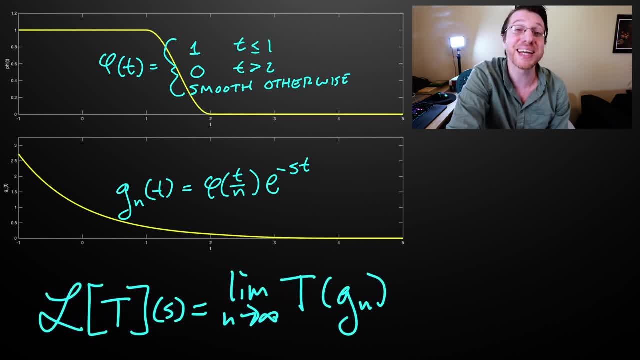 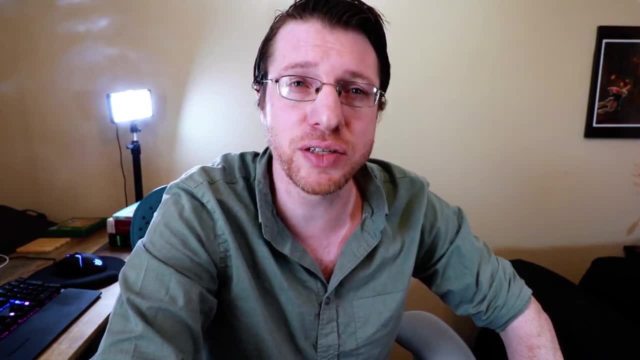 is given by the limit of the action of the distribution on this sequence of g? n's. So, with that definition, let's look at the Laplace transform of the delta function which, according to Nagel, Saff and Snyder, should be one. 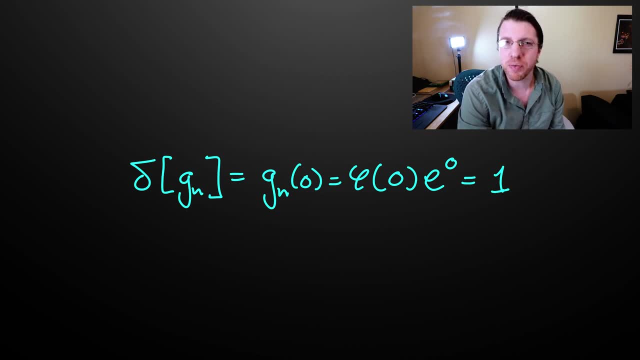 For each g n, delta of g n is equal to g n of zero, which is equal to phi of zero times e to the zero. but both phi of zero and e to the zero are one. Thus the sequence whose limit defines our Laplace transform.